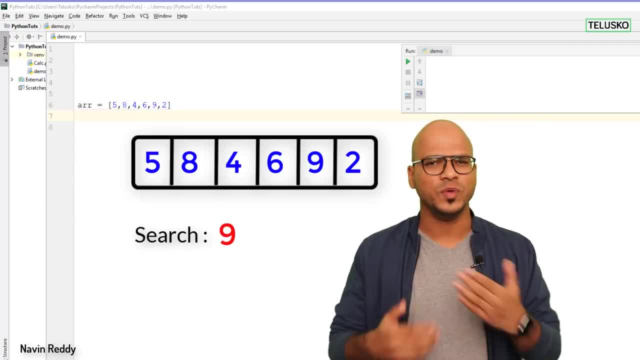 particular value and let's say you are searching for 9.. Now, how do we do that? So we do have certain functions in Python using which you can do that. But what if you want to do it by yourself? You want to do it manually using a loop. The general idea is: if you want to search for an 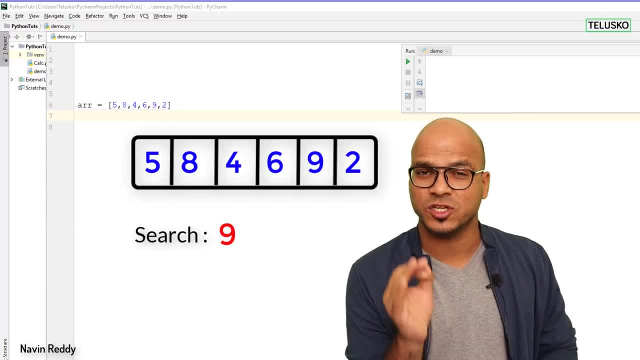 element. there are two scenarios here. The first scenario is the element which you are searching for is there in the list. The second scenario is the element which you are searching for is not there in the list. Let's go with the best scenario here. You are searching for 9 and 9. 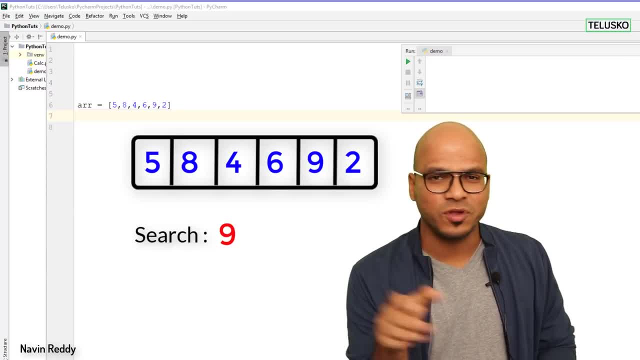 is there in the list right Now. how do we check? So we have to run a loop and you will check for each element. So let's say, if you are searching for 9, you will compare 9 with the first element of the list, which is 5 in this case. Since it is not matching, you will go. 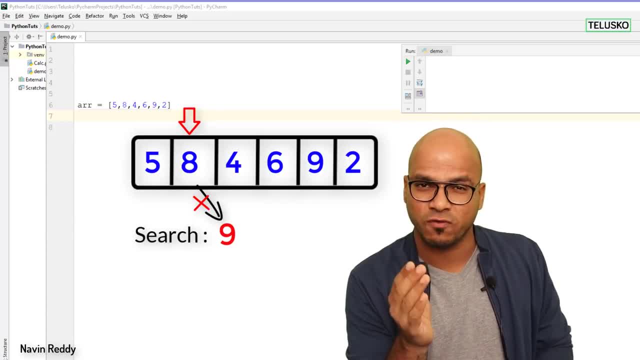 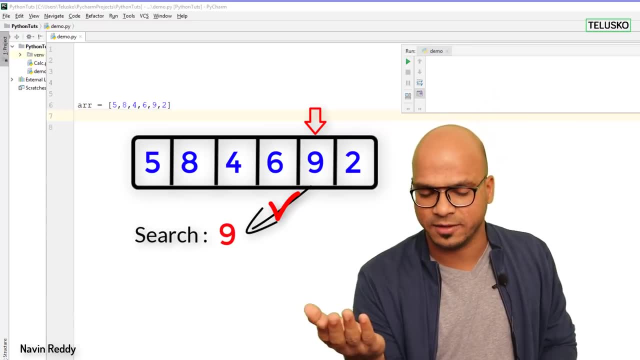 for the next element. We'll compare that. If this is not matching, you will go for the next element. That's what you do, And you will do this till you find the element right, Which is 9 itself, which is the fifth element in the array, with an index value. 4,, of course, or the list. 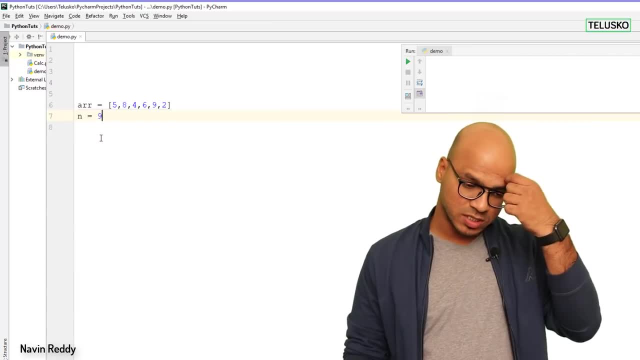 So let's do it. So the element which you're searching for is 9, right? So you want to search 9 from this list. In fact, let me just, instead of having the name as array, let me just list. 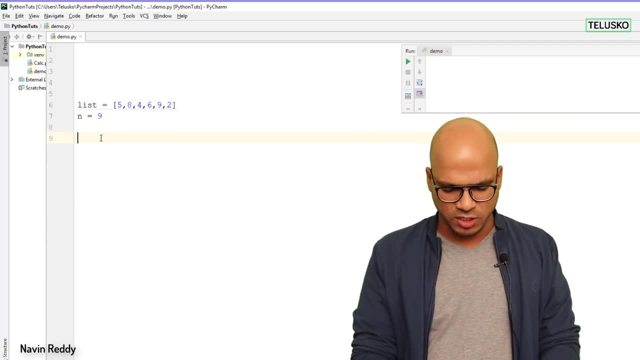 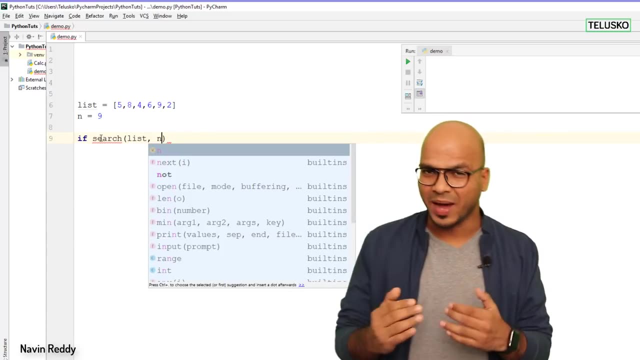 So we have a list and then we are searching for 9,. right Now you can use function. here You can say if search. So let's say, search is a function which we are implementing And in this search you will pass two things. So you will pass a list and you will also pass a value. 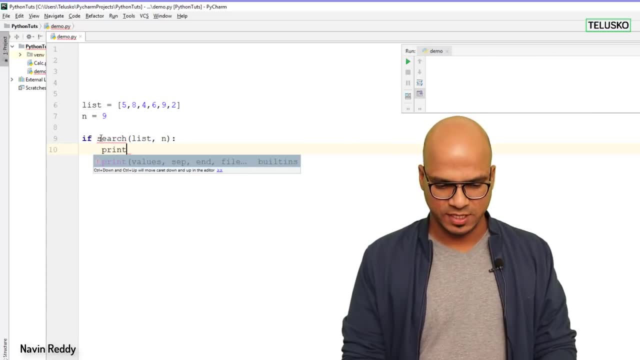 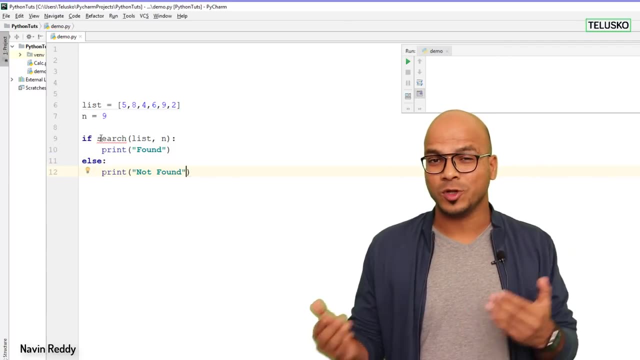 which you're searching for. If the value exists, you will simply print found. else you will print not found. So basically, if you're getting the value, you will print found or you will say not found. right Now, what is this search function? Is it inbuilt function? Of course not, You can. 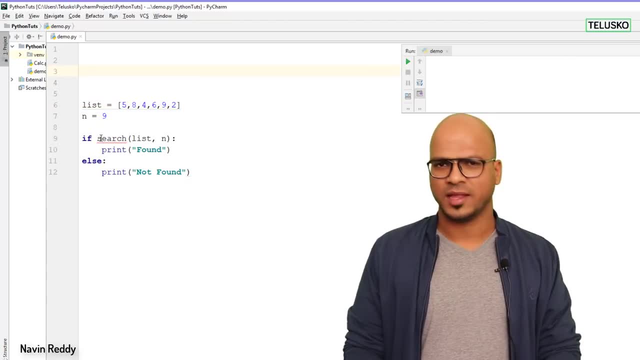 see, we are getting error there. So we have to define this function by ourself. And how do we define a function? It's very easy. You simply say def and the function name is search. And in this search you have to pass two values: You will pass a list and you will also pass a list. So 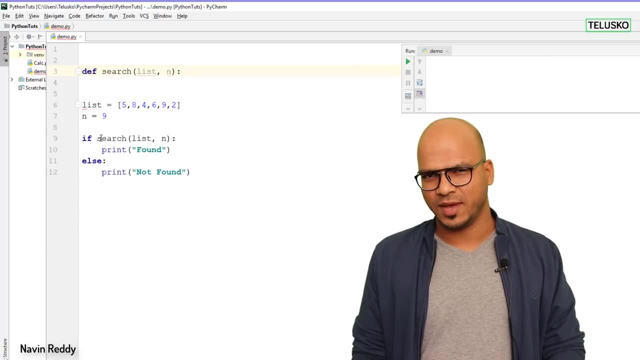 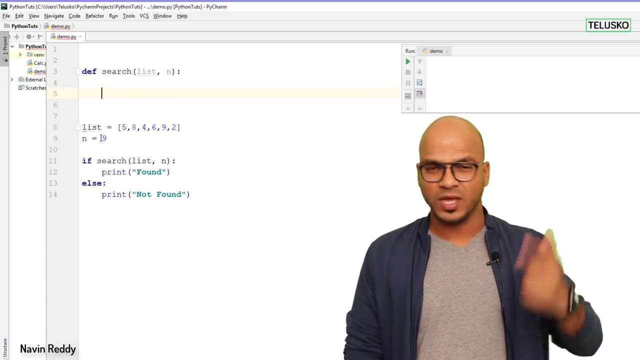 you will also pass the end value, which is n. You can change the variable name. as we know, We can have any variable name. Now, once you say you have this search function, what you'll be doing here Now? first of all, we have to use a loop right. We have to iterate from the first element to the 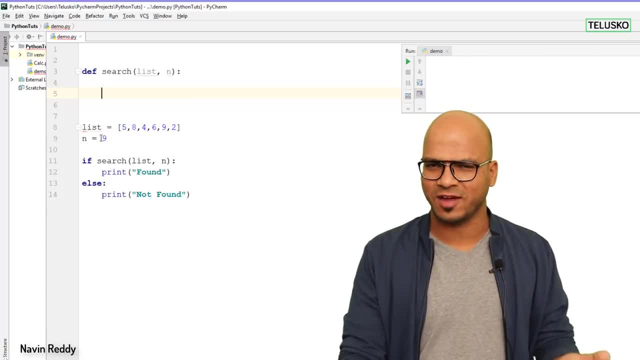 last element Now. we can use a while loop here. We can use a for loop here. We have multiple options. right, Let's start with while Now. in a while loop, you also need a counter, right, You can count the number of elements And the way you can use a counter by saying i. normally we can. 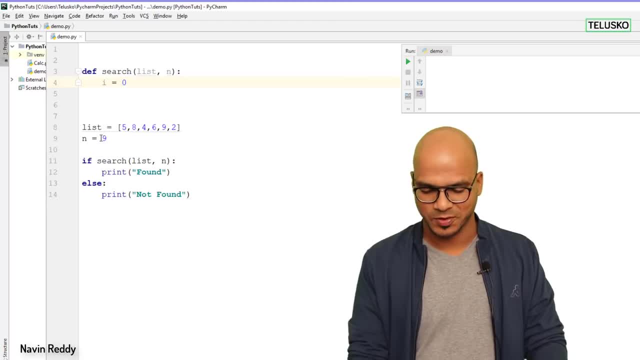 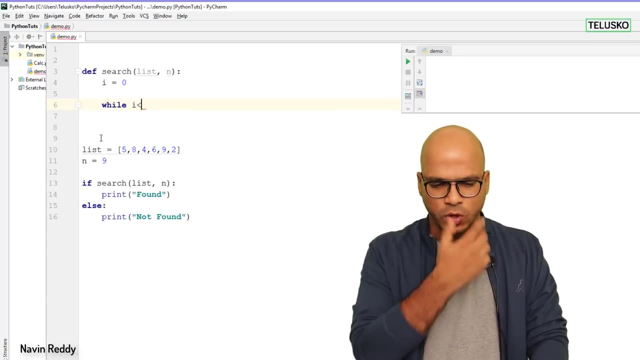 use any variable name. but i makes sense when you have a counter for the loop, Right. So we are saying i is equal to zero, And the next thing we need is let's use a loop here. So we will say while, and we have to go till where? So you have to go to the last value. So how do you? 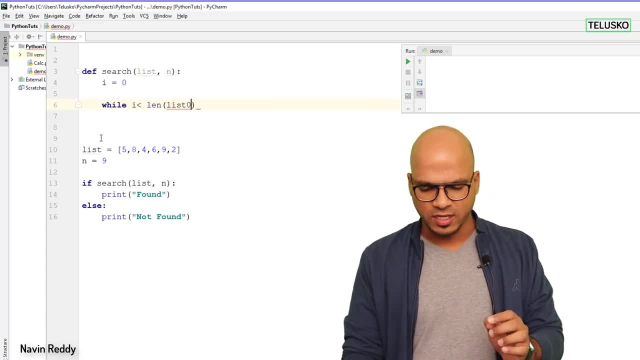 know the last value, So you will simply say length of list. Now, if you can observe, I'm using less, okay, I'm not using less than equal to. The reason is this is a list. right, Index value will start. 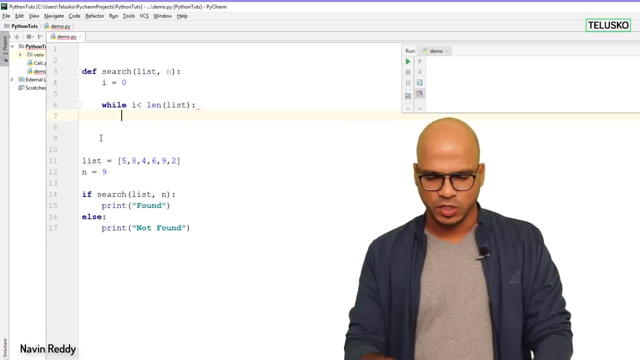 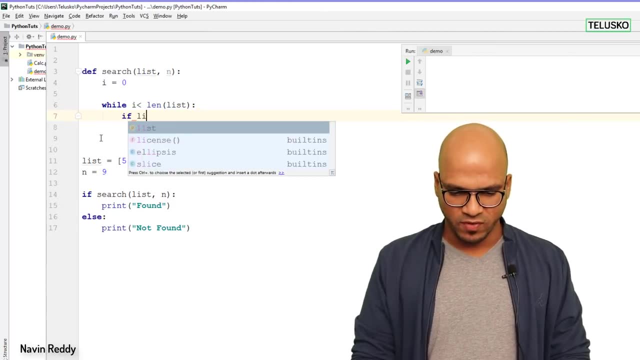 with zero. So let's keep it length of list And then you will simply check for each value. So you're going from the first element to the last element, right? You're using a loop here. So you, if the value in the list you will use a counter i is equal to n. okay, So the moment you find the 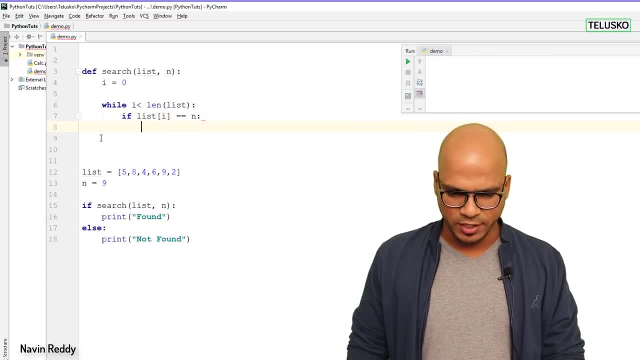 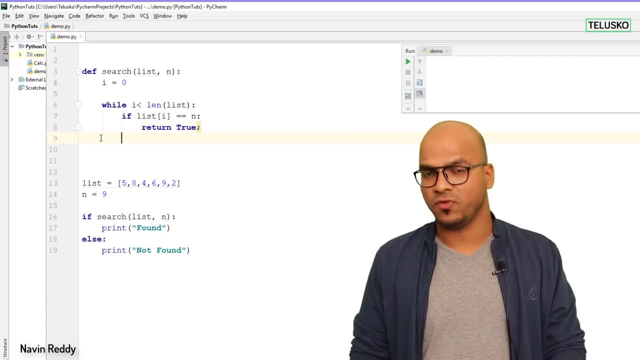 value, you will stop it right. So if it is equal to n, you can use: oh, how do we say that we have found it? So we can simply return true. So we can simply return true the moment you find it. 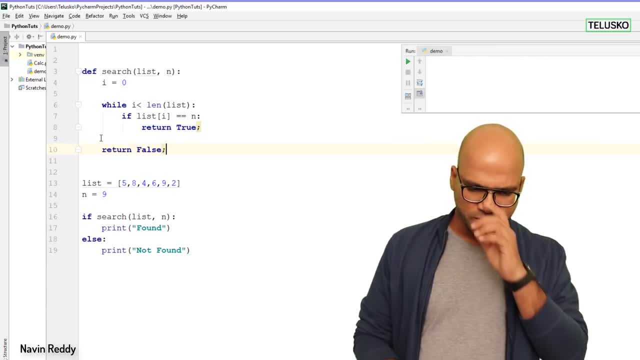 And that's it. At the end, you will return false. So what we're trying to do here is: the moment you find the value, you will simply return true. Otherwise you will return false. That's it. That's the code we have written here. Now will it work? So what exactly we are doing is: 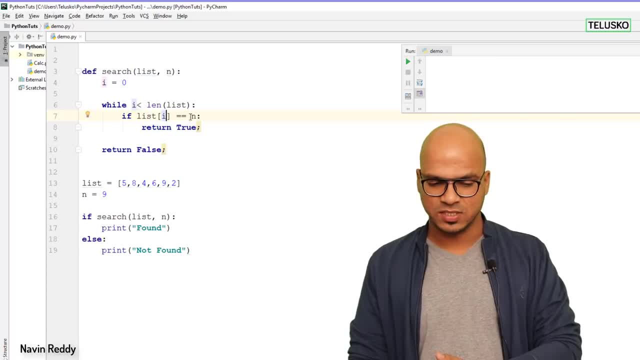 we are comparing with the each value. If this is matching with the list, or the value which you're searching for is in the list, it will simply return true. Otherwise, after the loop ends, it will return false. right, That's what we are doing. Let's verify if this is working. 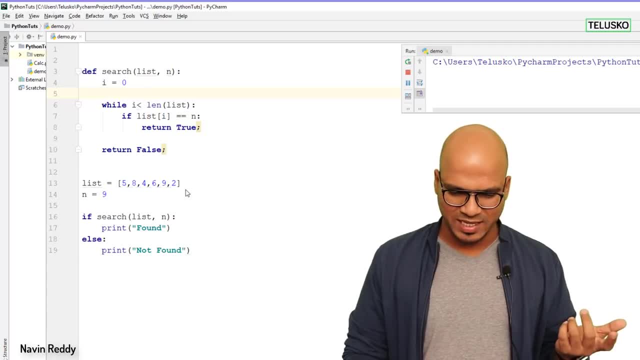 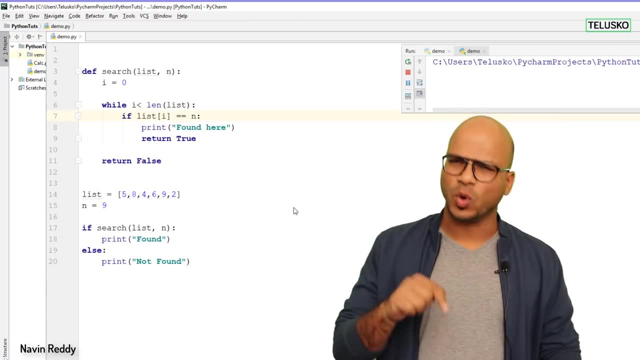 Let's right click and say run demo And oh, we have not got any output. but why Is it? because I'm using semicolon. Let's remove that. Let's print something here, Let's print. It is not even going in this inside the list. You know why? Because we are not incrementing the while loop. 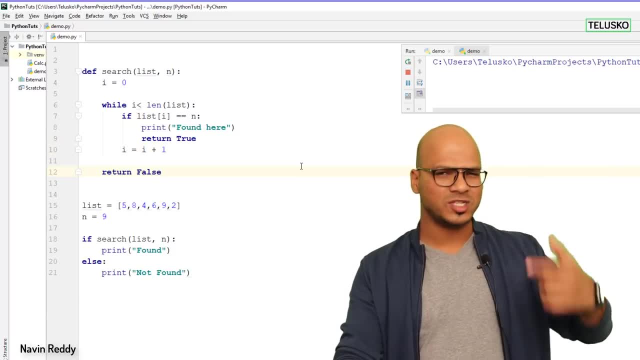 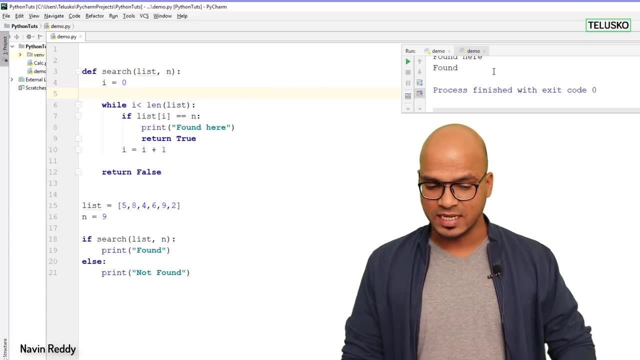 We missed that. We have to say i is equal to i plus one, right, So we are not changing for the value for the. i Just keep comparing with five. We do not do that, So let's increment. So we have done that. Let's run this code And you can see. it says found and. 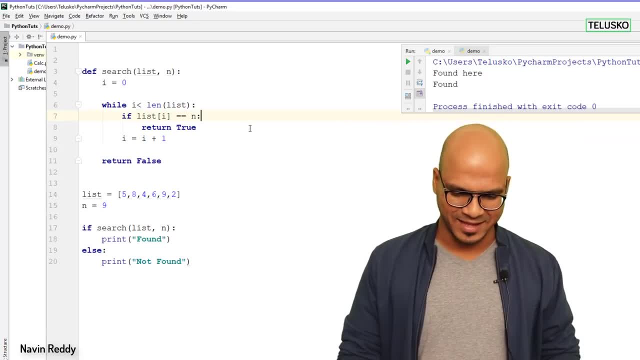 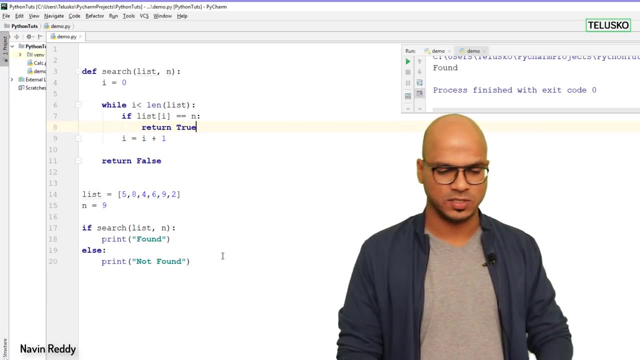 found here. So let's remove this found here from here And now let's verify again: Is it working? So, yes, you can see. it says found. The value is there, right, The value is there in the list. What if I give a new value? What if I'm searching for 10? And you can see we don't have 10 in the 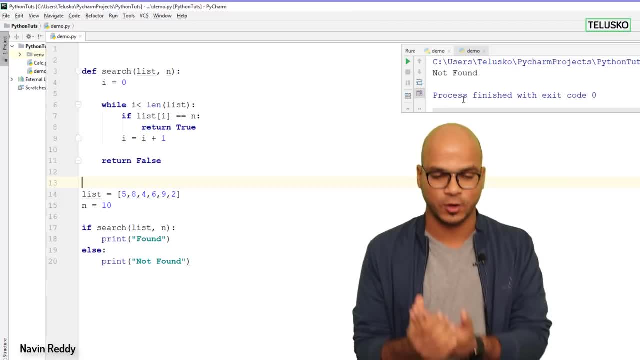 list And the moment you run this code, you can see it says not found. So we got the code. So what we are doing is we are comparing the value with each value. The moment you find the value, you will simply return true. 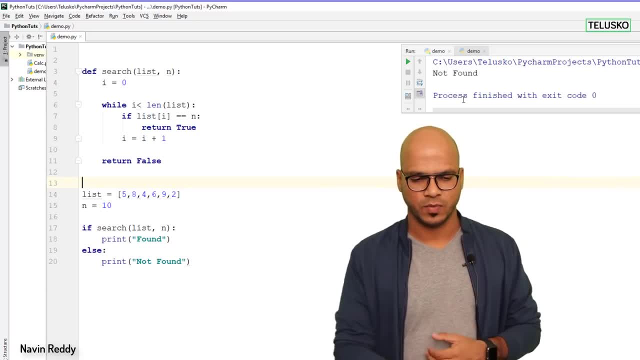 Otherwise, at the end, if it is not returning, it will simply return false right. This is where it is happening. But we still have one problem here. You can see I'm simply printing that we have found the value but we are not saying where it is right. We have to also maintain the position. 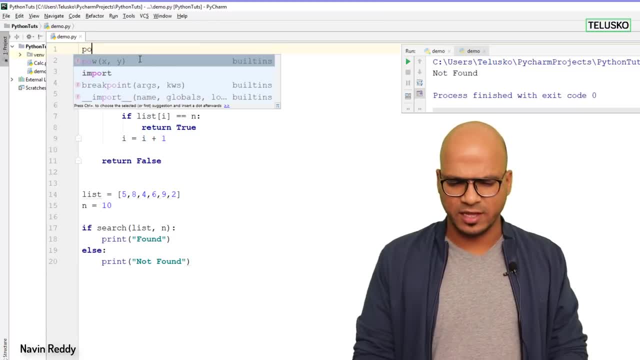 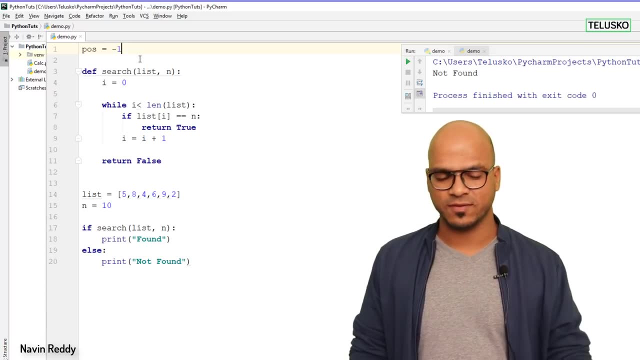 and we are not doing that. So what I will do here is I will say: let me take a variable which is pos, and by default the value for pos will be minus one, because norm index will start with zero. When I say minus one, that means we have not got the value, so we can actually debug it. 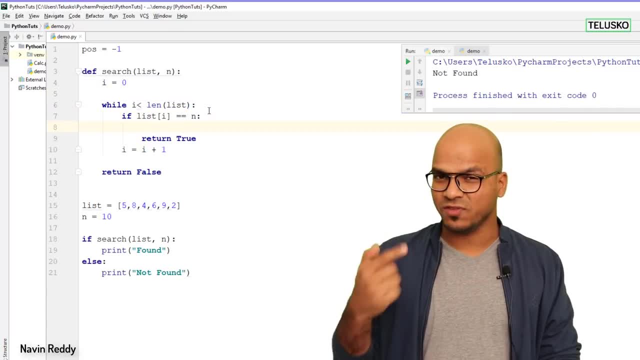 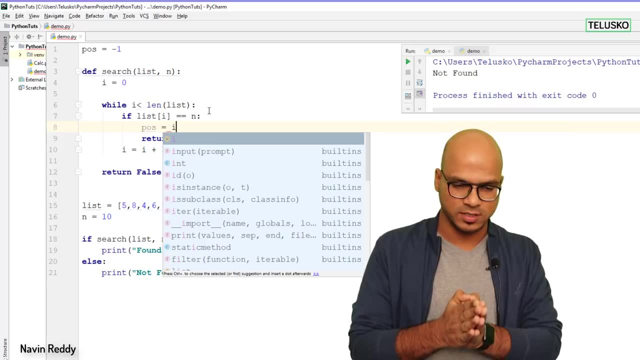 But time, let's skip it. Minus one, And here, the moment you find the value, let me also reserve that position of i. okay. So whatever value of i is, I will save that in pause. But there's one issue Now. 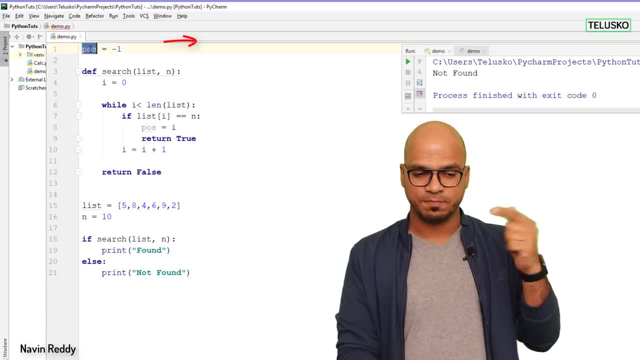 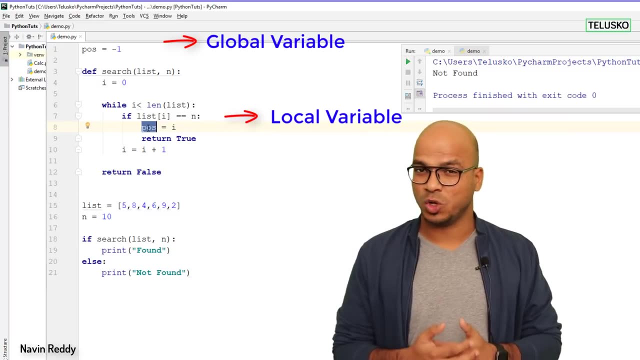 if you have seen my video on global variable and local variables, this pos is a global variable, right? And this pos here inside the function becomes a local variable And when you change a local variable it will not impact the global variable, right? Because I want to use that. 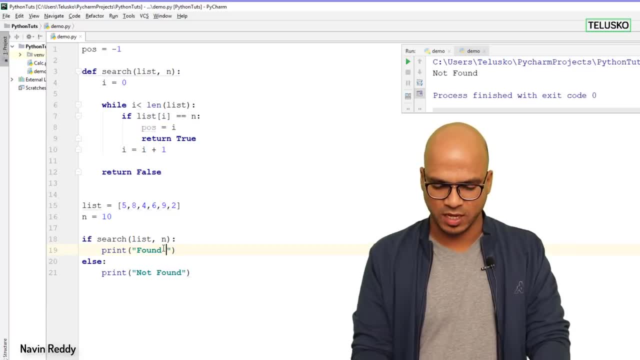 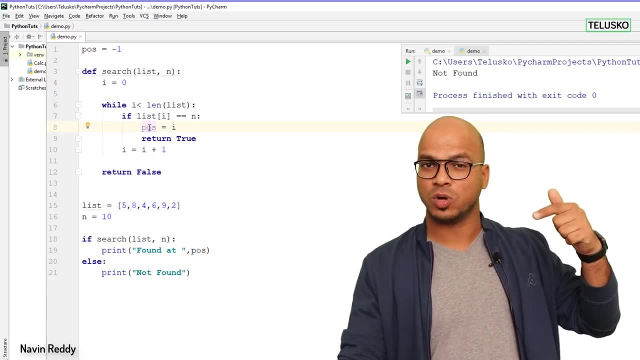 position outside the function. So I want to use it here. So I will say found at and I want to print the position as well. The problem is when I change the pos value here, it is changing the local variable, not the global variable In order to access the global variable. 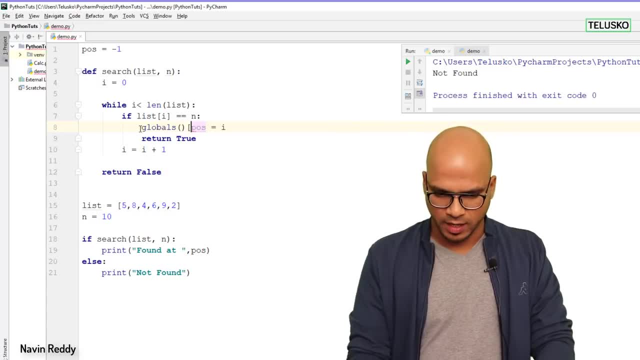 if you remember, we simply use a global as a function and then we can give this pos as the, because we can have multiple global variables. right, We have to mention which global variable we're talking about. So there's pos in this case. Now it seems good, I will simply run this code and: 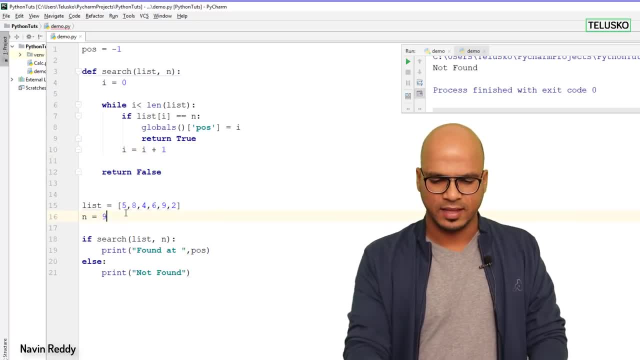 you can see it says: oh, it says not found because we are searching for 10.. Let's go back to nine and let's run this code And you can see it says found at. and let's run this code And you can see.